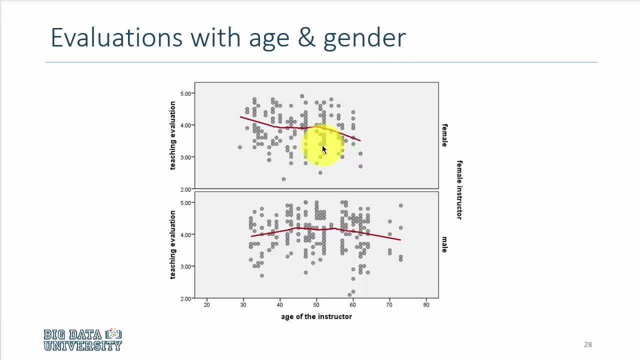 from hollow circles to square circles. The bottom panel is male, the top panel is female. I've changed the circles to filled circles- gray colored filled circles- and, more importantly, I have added lowest lines, which are sort of regression type lines, to see that for female instructors we see. 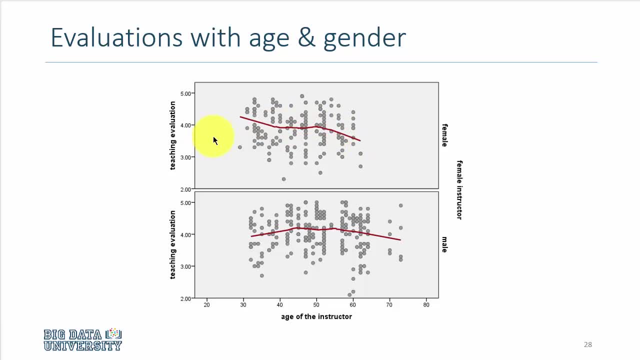 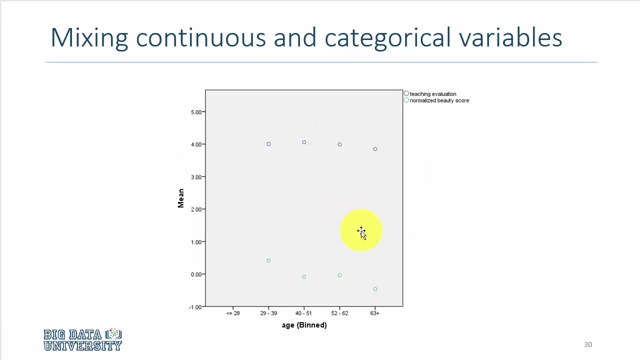 sort of a downward sloping curve of teaching evaluations as age increases. But we don't see the same declining trend for males. It's sort of a rising trend with age, then it sort of levels off and then eventually it declines. In this particular graphic we have the same type of 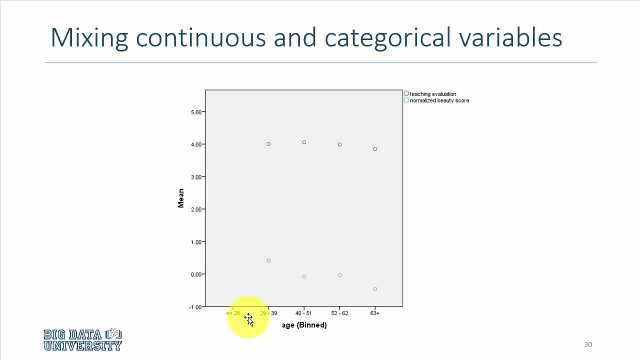 information, but we have changed the age variable from being a continuous variable to an ordinal type of variable where age is now in different brackets: less than 28 years of age, 29 to 39 years of age, 40 to 51,, 52 to 62, and 63 plus. In addition, the color of these circles is not representing. 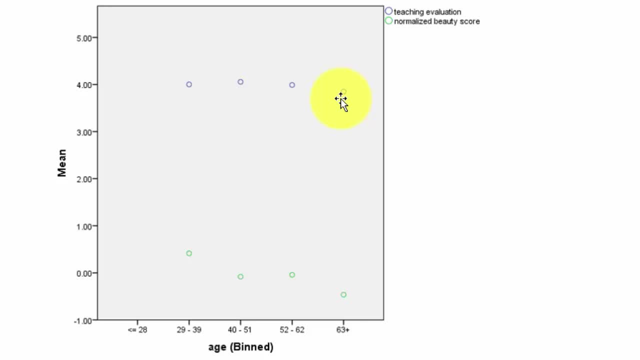 males or females, but in fact it is representing two different variables. The blue color is the average teaching evaluations by age and the green color circles are the normalized beauty score. You could see that the normalized beauty score prepared to decline with age and the teaching 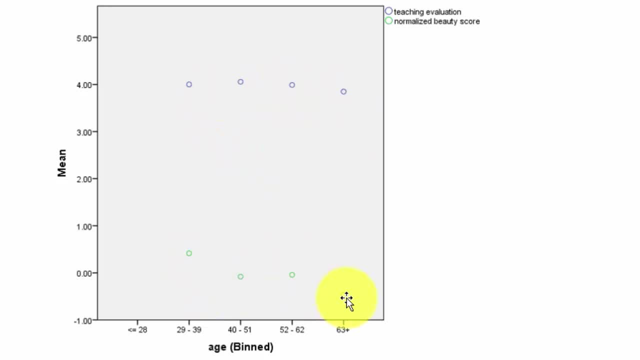 evaluations do not have the same downward sloping impression here, Since we did not have any instructors under the age of 28, we have a redundant category in the in the graphic. If we were to be using scripts, which is an option available with SPSS. 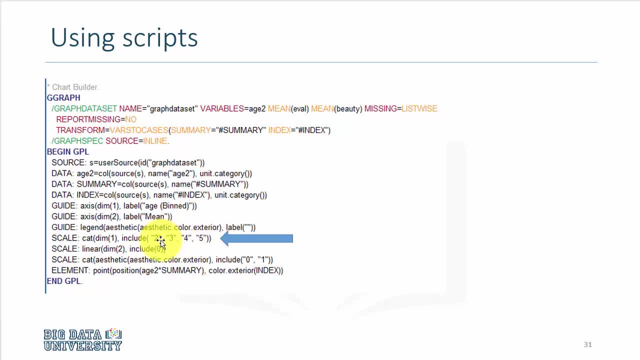 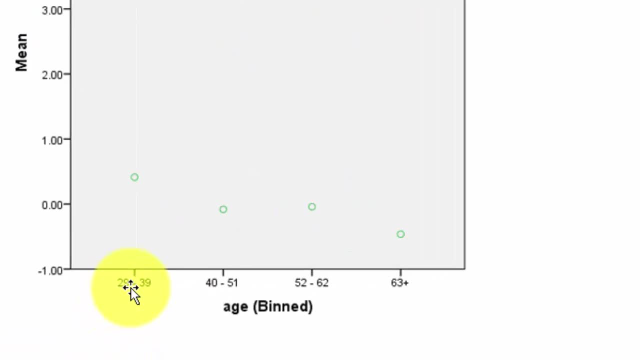 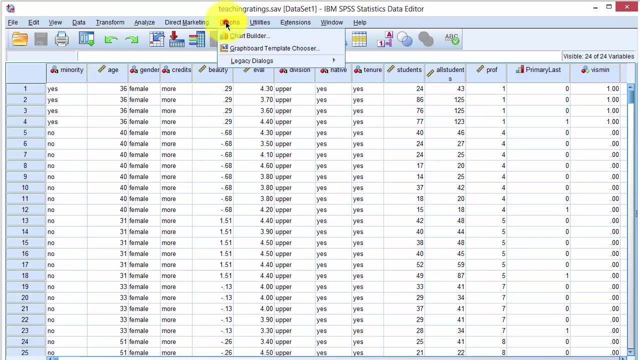 we can actually remove the first category, which I have done here, and redrawn the same graphic to and now you see here that the less than 28 years of age category has been removed from the graph and there is no redundant information in the graphic. In SPSS we click on graphs: chart builder. 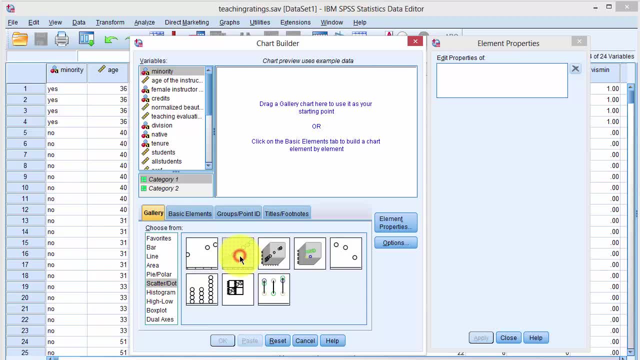 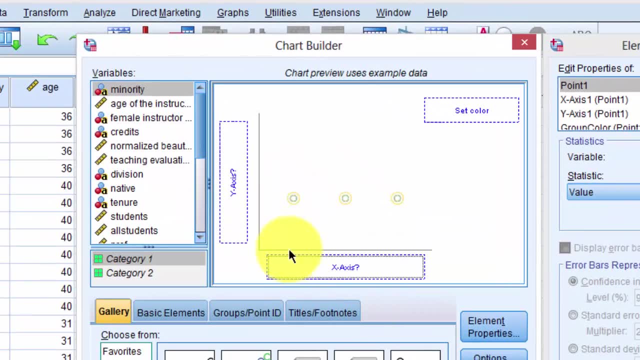 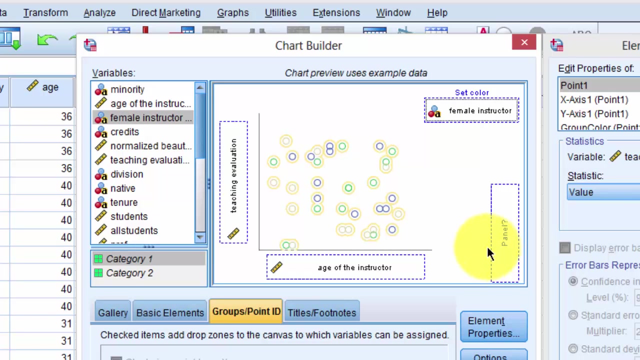 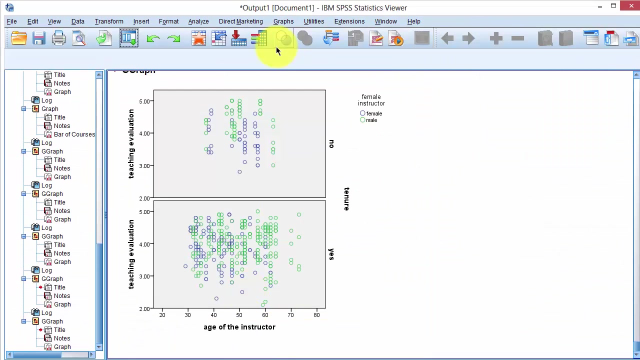 and select scatter, second template, draw it to the canvas and now we will populate this template. We put the age on the x-axis, teaching evaluation score on the y-axis, the coloring is set by gender and we add the additional dimension of tenure to the panel. Click OK and here's the resulting graphic. To add the regression line, we double. 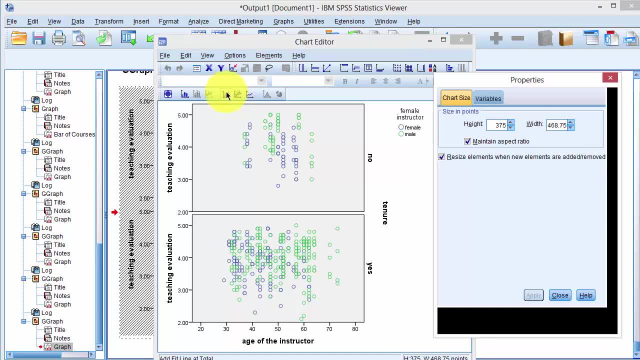 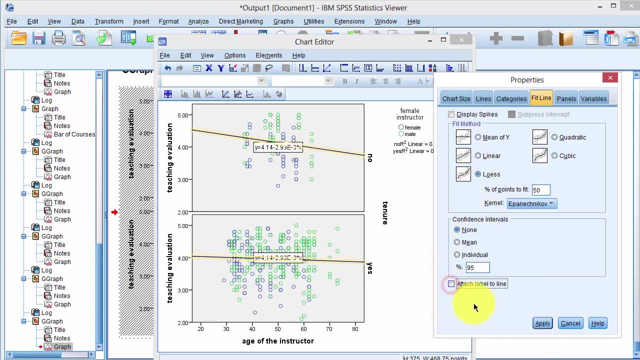 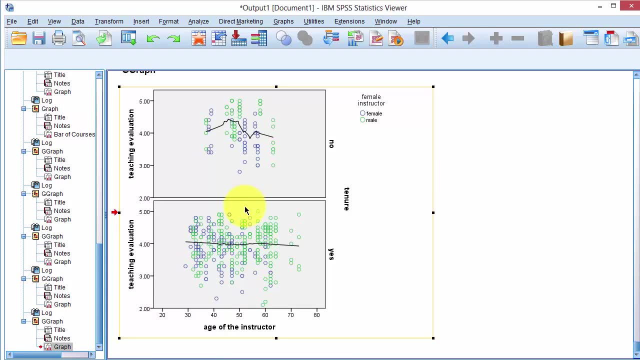 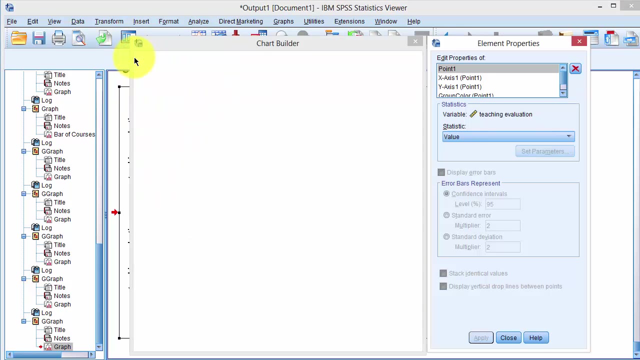 click on the chart and then click on regression line and press enter, Pick lowest option and deselect, attach label to line and click on apply and close the editor and we have the lines drawn. We can change the color by double clicking on the line To remove tenure. we go back to chart builder dialog and remove the row and panel variable. 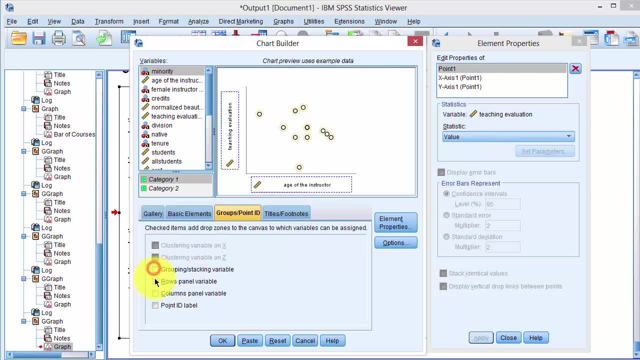 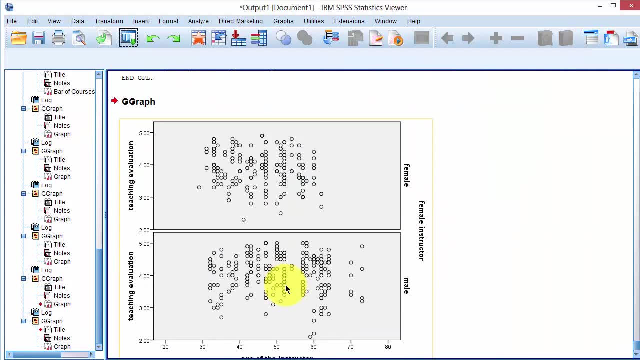 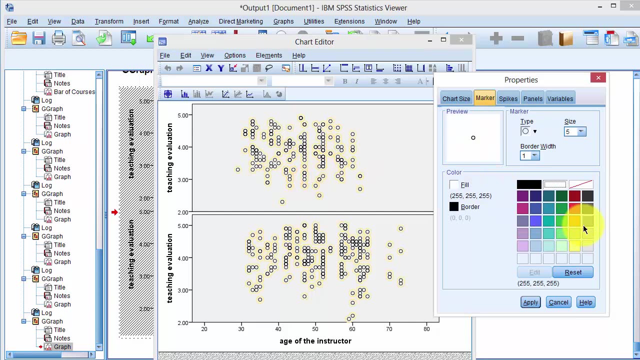 and remove the grouping stacking variable and instead select the gender as the panel and click okay. and now we double click on it to edit this graphic. We select first the circles and click on fill and select gray color and for border a darker shade of gray, say apply, and then click on regression line, click on lowest deselect. 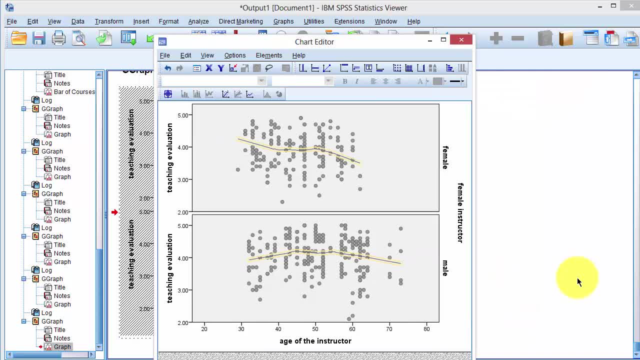 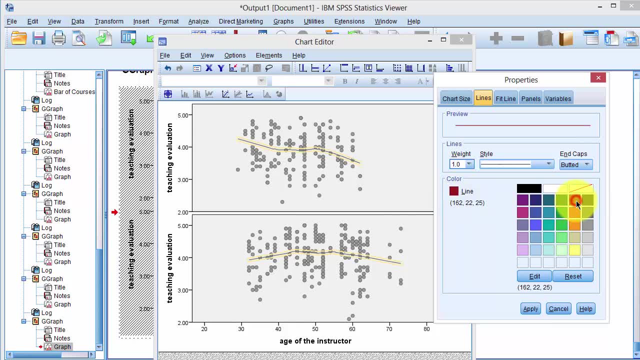 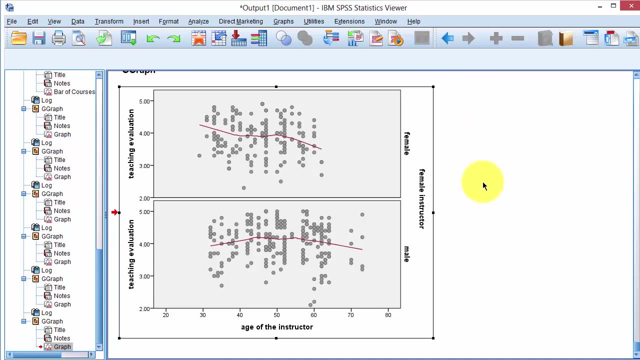 attach label to line. Click apply To change the color of the line. we double click on line and select color and select a different color. say apply, close the dialog box. and here's the scatter plot between age of the instructor and teaching evaluations with a regression type line fit to it. 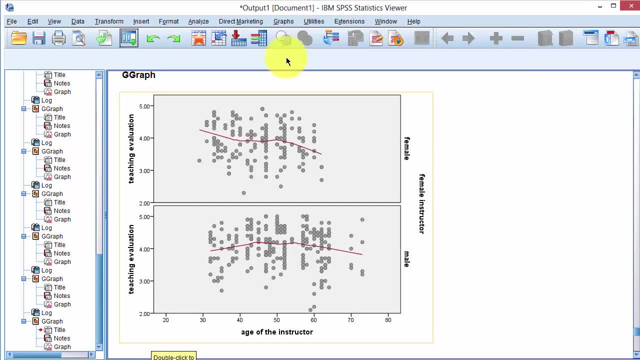 Now let us try to generate average teaching evaluation and normalized beauty score in the same graphic. We will use a categorical variable for age and instead of using a continuous age variable, we will use a categorical variable for age. So we click on chart builder and we click on scatter dot plot, and this is the right. 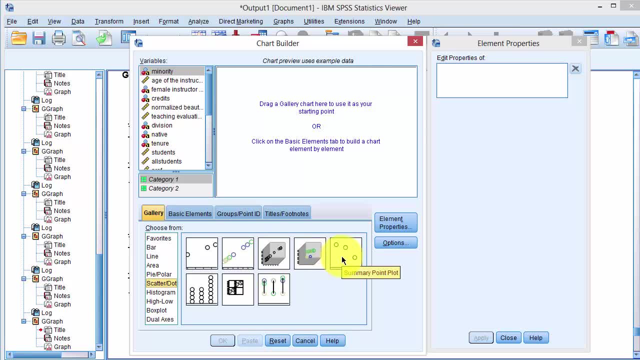 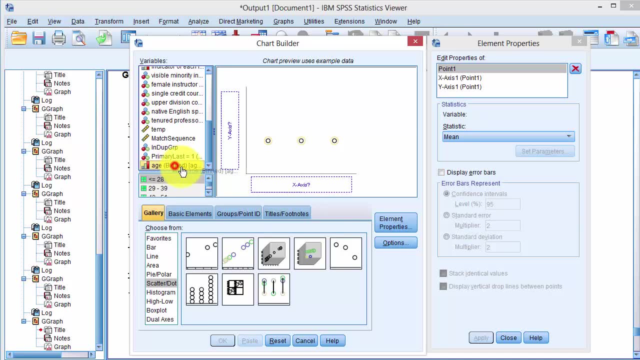 most option, which is summary point plot data that we want. so we drag it up there and on the x-axis, we will put the variable age, which is binned. age is binned into different categories and we now select the two continuous variables being the normalized beauty score and the 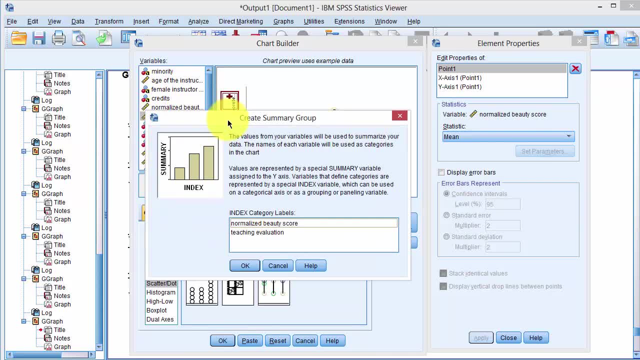 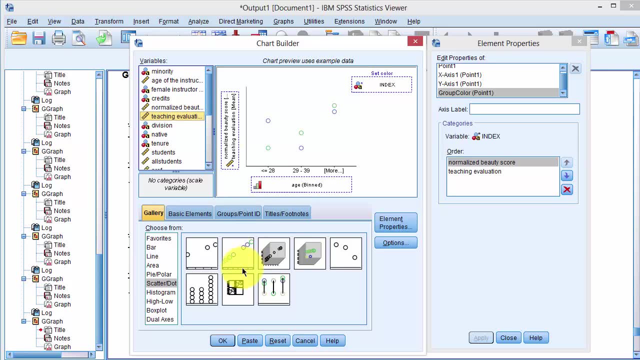 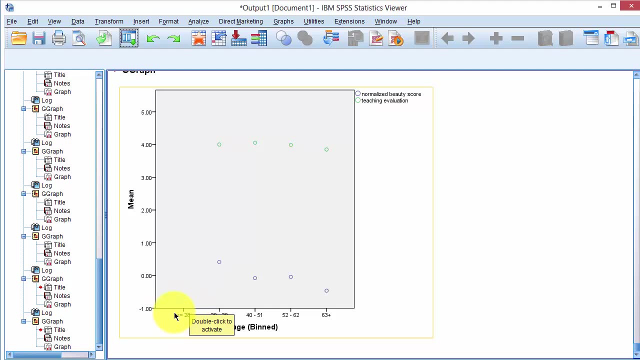 teaching evaluation score and drag them to the y-axis and we get this notice from SPSS and we just say okay, and that's pretty much it. We click okay and the output should appear. Notice this redundant category at the end, which you can remove using the script option.